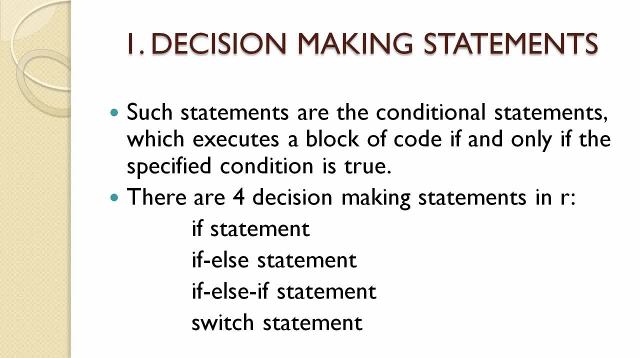 contain some conditions with along with them, and executes a block of code only if the condition is true and execute some another block of code only if the condition is false. So in decision making statements there are four statements. they are: if, if else, if else, if and if box. 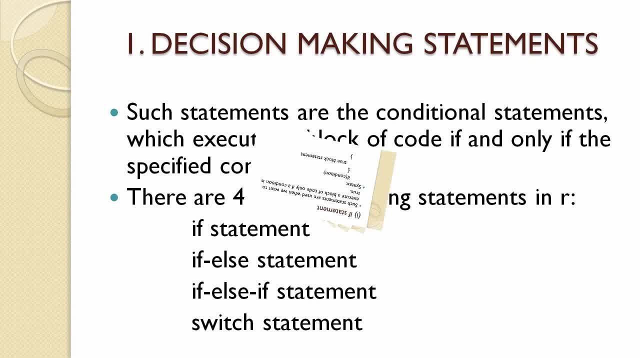 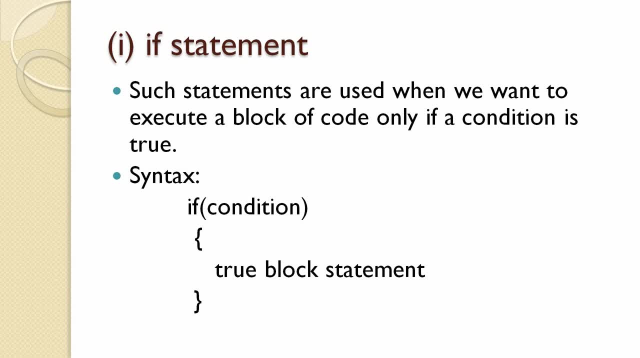 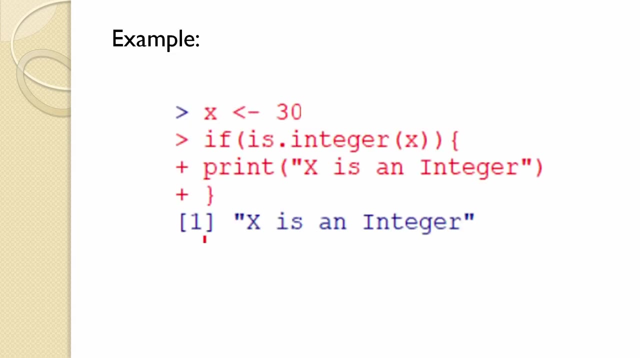 if and switch statements In simple if or if statements, we would execute a true block statements only if this condition is true. In syntax we can see that if followed by parenthesis which contains an expression or condition which needs to be true to execute the true block statements within curly braces, If we come to an example, we have assigned a 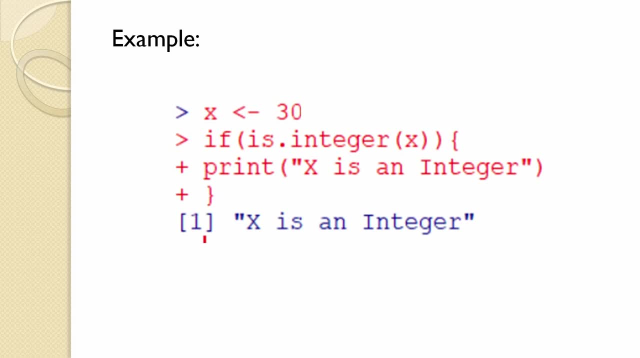 variable x with a value of 30 and we want to check whether it is an integer or not. Thus we have written a statement that if parenthesis is integer of x, which means that if the variable x contains an integer value, then it would execute the command print. x is an. 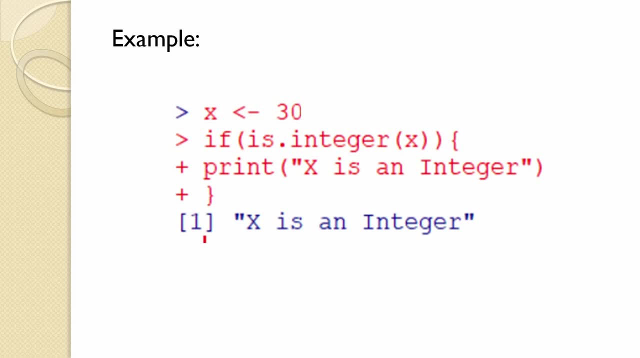 integer, As we know that 30 is a value of integer type. thus the condition is: dot. integer of 30 is a value of integer type. So if we come to an example, we can see that if the variable x contains an integer of x is true, Hence the output will be: x is an integer. 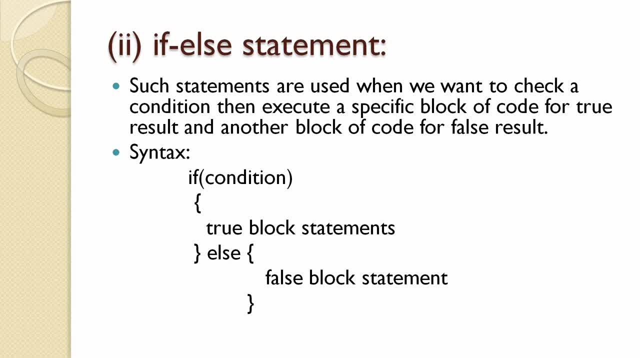 The next one is if else statements. Such statements are used when. when the specified condition is true, then we would execute a some other block of code, and if the condition is false, we want to execute another block of code In syntax, if we can see that. if contains the 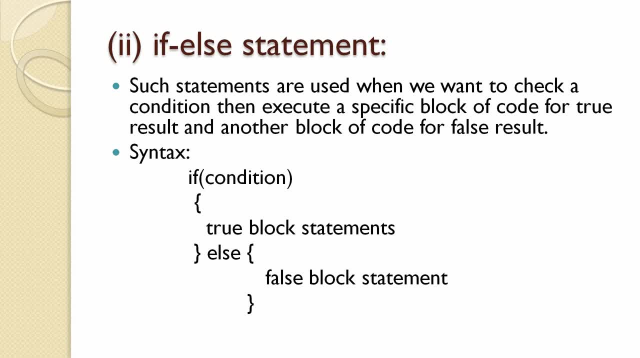 condition or expression. and in parenthesis, if the condition is true, then the true block statements will be executed. But if the condition is false, then the true block statements will be executed. But if the condition is false, then we would move on to the else block statements. 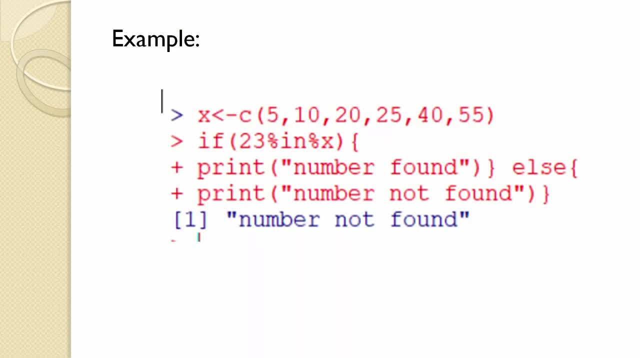 which contains false block statements. If we come to an example, we have assigned a variable x with a vector of elements 5, 10,, 20,, 25,, 40 and 55. And we are interested in checking whether 23 number is present in x or not. Thus we have specified a condition: 23 percentile. 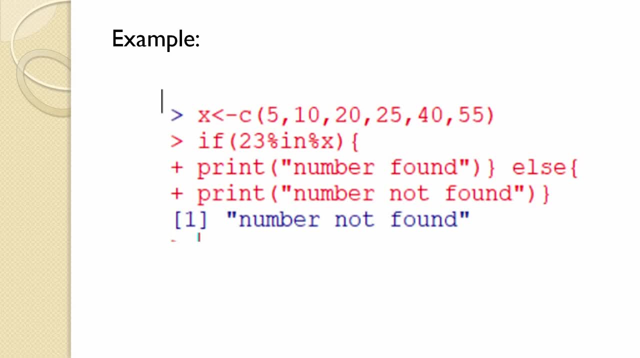 in percentile x, which checks whether 23 number is present in x or not. If this condition is true, then the command print number found will be executed. But if this condition is false, then we would move on to the else block which contains a command print. 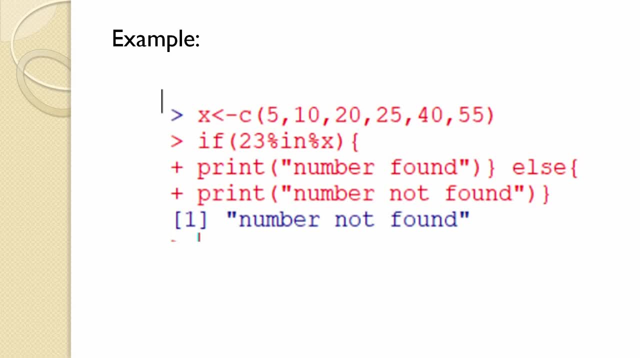 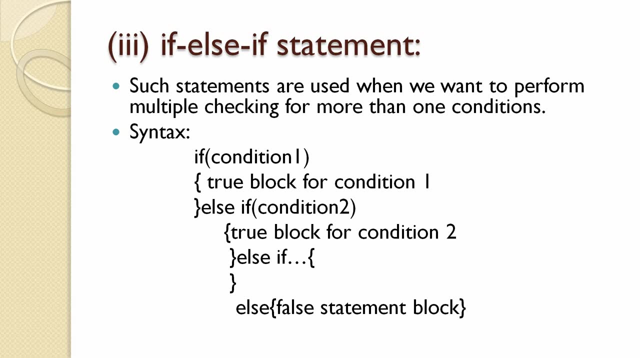 number not found, As we can see that the number 23 is not present in the vector x, so the result will be number not found. The next statement is if else, if statement. These are the statements which are used when we want to perform multiple checking for more than. 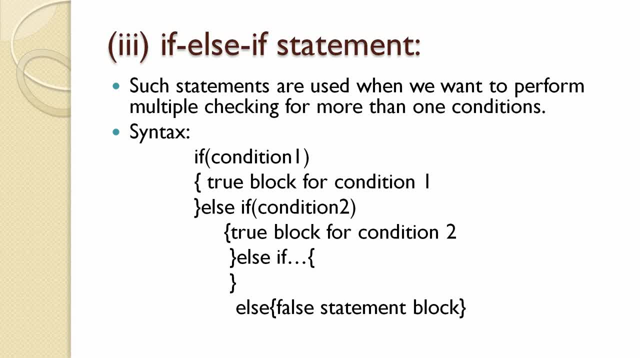 one condition. For example, if in syntax we can see that if condition 1.. If this condition 1 is true, then true block statements for condition 1 will be executed. If condition 1 is false, then we would move on to the else block which contains another if with condition 2.. If this: 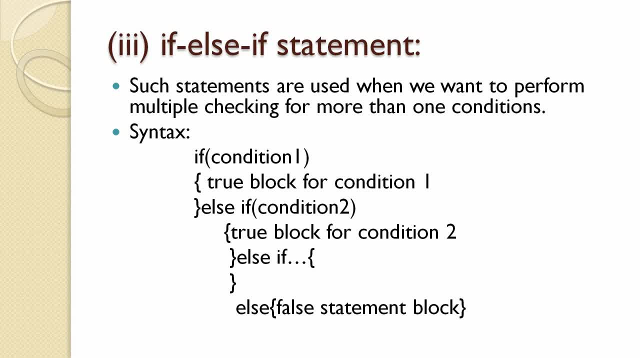 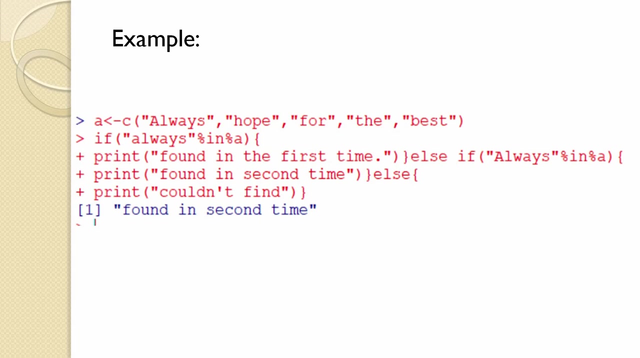 condition 2 is true, then the true block statements for condition 2 will be executed. But if this condition 2 is false, we would again move to the else block. Let us see an example Here. vector a contains the string type values which are always hoped for, the. 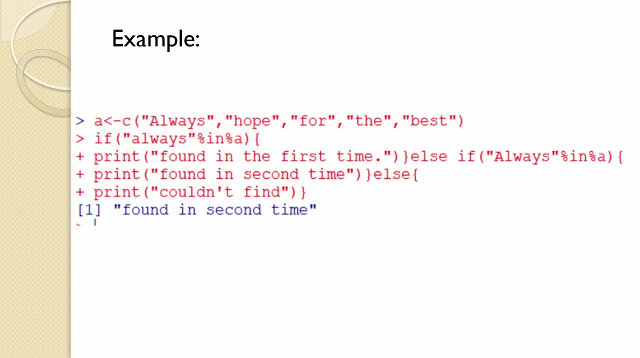 best, And we are interested in checking whether the word always hope for the best, Starting with small letter a, is present in the vector a or not. If this condition is true, then we have given a command to print found in the first time. If this condition is false, 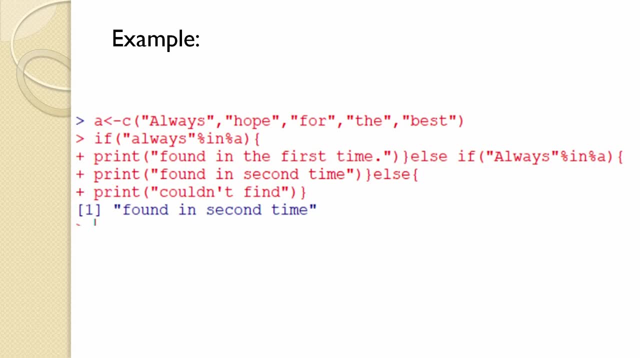 we would move on to the else block, which contains another if condition, which says that the word always with capital, a, is present or not in vector a. If this condition is true, then we would move on to the command print found in the second. But if the second condition is again false, then we would move on to the else block that contains 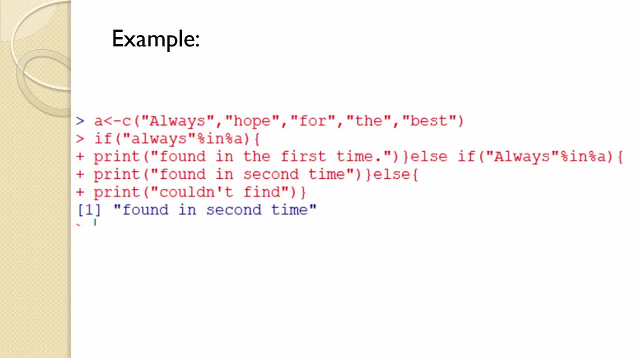 the false statement to print couldn't find. Thus, as we can see that the letters always starting with small a is not present in the vector a. Thus the first condition is false. Thus we move on to the else block of the first condition. Here we can see that the word always starting with capital, a, is: 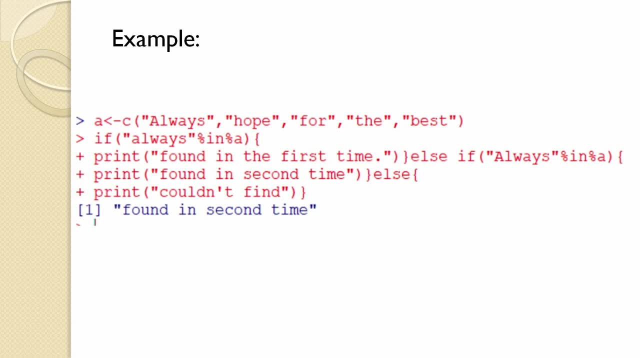 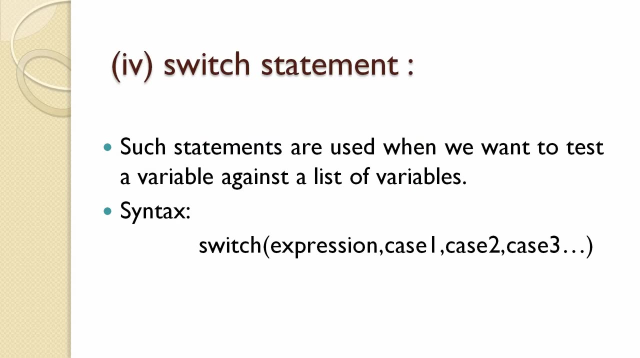 present in the vector a. Thus this is a true statement. Hence we would get the output found in the second time. The next statement is switch statement. These are the statement which are used when we want to test a single variable against a list of variables. In syntax, we can see that switch is the keyword. 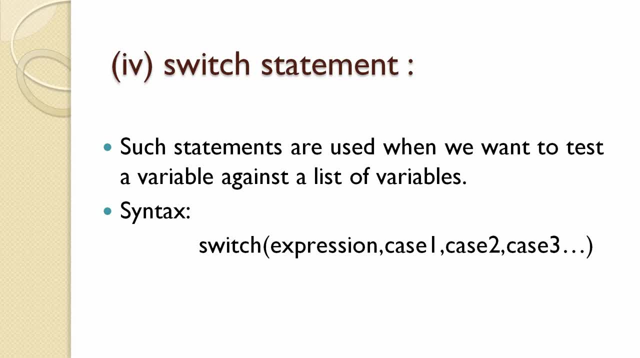 in which first we have to specify the expression or condition of the variable And we want to check the expression. Myth 3 of this statement is to print the25 number case of the values with case1, case2, case3, End, so on up to End cases. 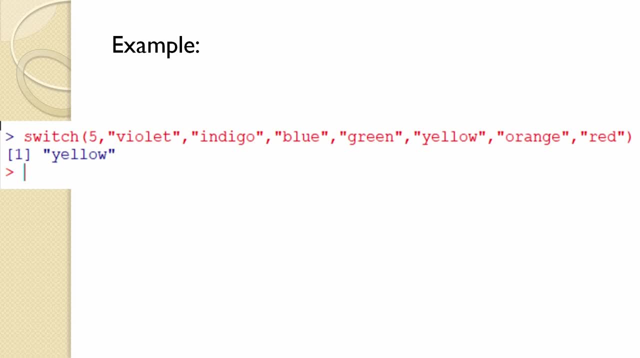 If we say an example, we have written switch 5.. Which is a number against the variables which are of string type: violet, indigo, blue, green, yellow, orange and red. This statement means to print the 5th number case of the given case. 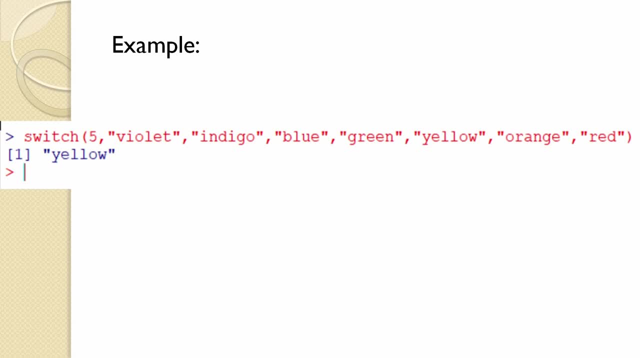 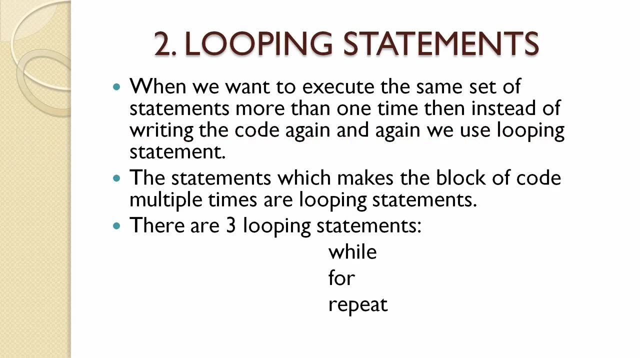 here the 5th number case is of string yellow. Thus the output is the alternative value here: yellow. the next control structures are looping statements. when we want to execute the same set of statements more than one time, instead of writing the code again and again, then we use the looping statements in R. there are three. 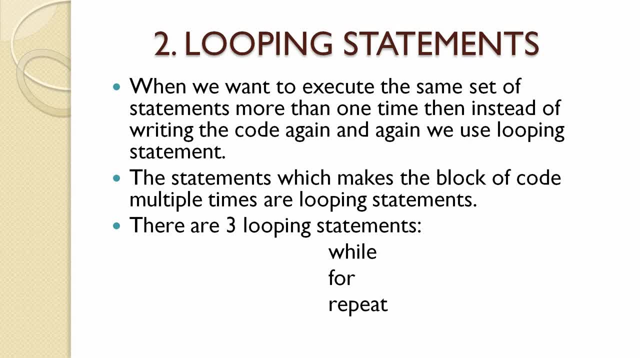 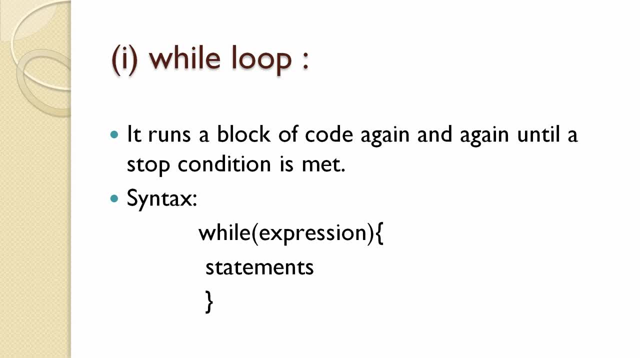 types of looping statements. they are while for and repeat loop. let us know about while loop. it is a loop which runs a block of code again and again until a stop condition is met. in syntax, we can see that while, which contains an expression within the parenthesis and a block of statements which are to be 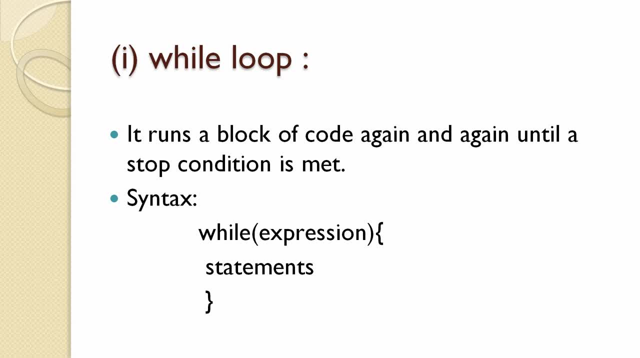 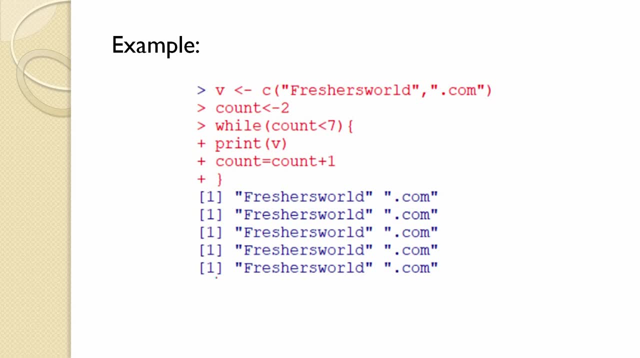 executed when this expression is true. if we see an example: we have defined a vector V with elements precious world and dot-com and also specified a variable named count with value 2, and we have written a while statement while count less than 7, which means count should be less than 7. then the statements which are written: 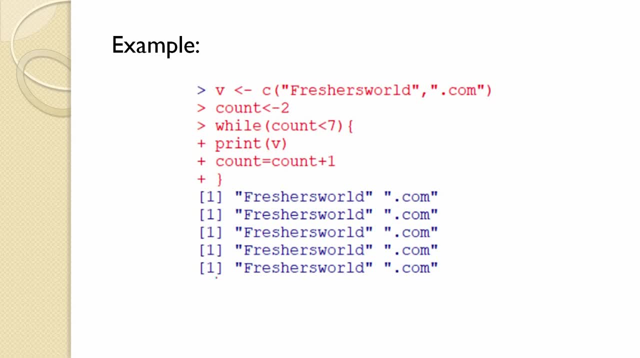 inside the while loop will be executed. in the while loop the statement is print V. we have to print the vector V and count equal to count plus 1 and increase the value of count by 1 every time the program enters into the while loop. here first the value of count is true, which means 2 is. 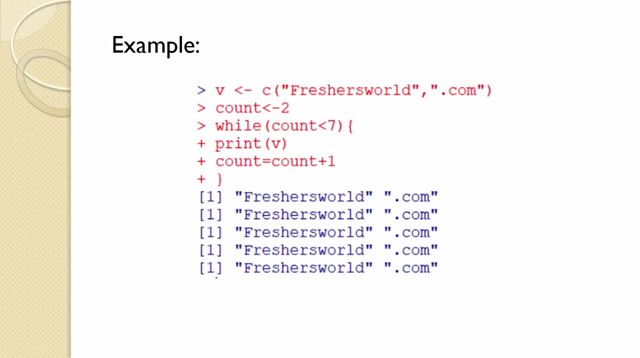 less than 7. this is true. so we enter into the while loop and print V, which is freshersworldcom, and increase the count by 1, which means that new count value will be 3, and we would again check the condition whether count is less than equal to 7 or not. here 3 is. 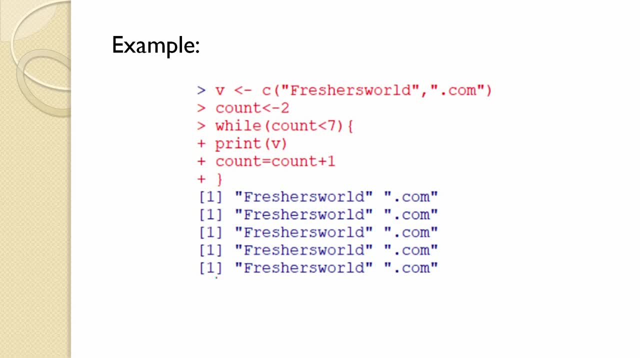 less than 7, which is true. thus we again come into the while loop and print V, which is freshersworldcom, and increase the value of count by 1, which means the count value will be now full. this is really bad and we can get one. 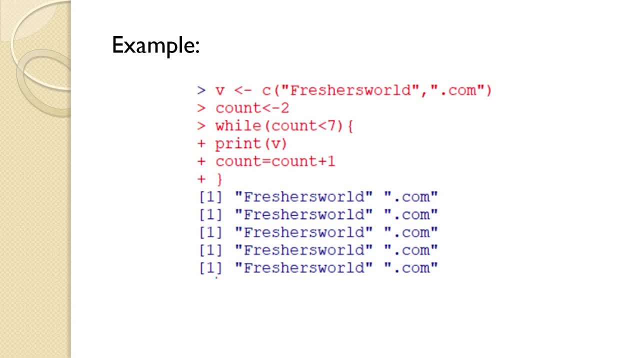 4. again, we would check the condition whether 4 is less than 7 or not, which is again true. thus we enter again into the while loop and print freshersworldcom and increase the count value by 1. now the count value will be 5, which is, which again satisfies the condition count less than 7. 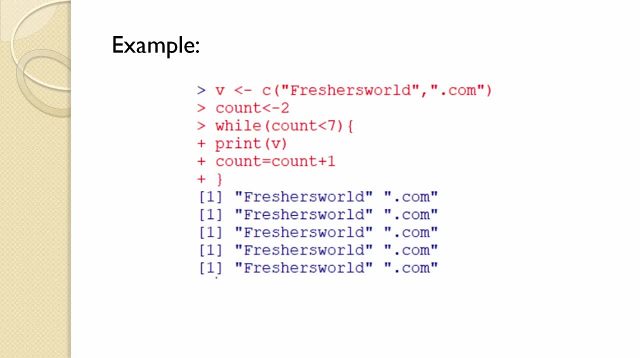 thus we again enter into the while loop and print freshersworldcom and increase the value by 1 of count, then the count value 6 is again less than 7, which is true again. thus we again print freshersworldcom and increase the value of count by 1, then count value becomes 7. now is 7 less than. 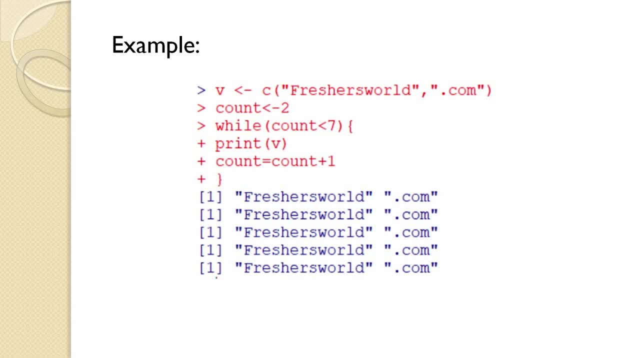 7. no, as 7 is equal to 7. thus the condition count less than 7 becomes false and the program exits the while loop. thus we get the output of freshersworldcom: repeat, repeated five times. hope you all understand the concept of while loop. let us move on to the next. 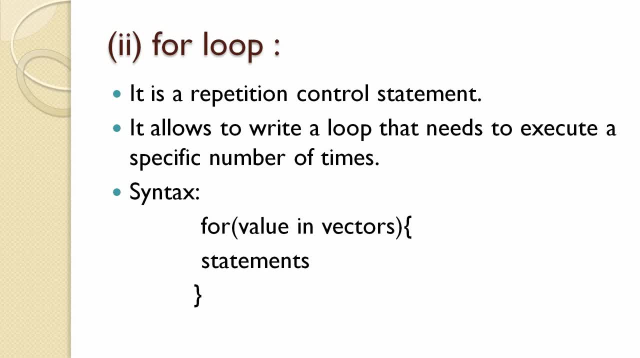 concept for loop. it is a repetition control statement, for loop is also known as a repetition control statements, which allows us to write a loop that needs to be executed a specific number of times. in syntax we can see that we have written for in the parenthesis we have given the condition. 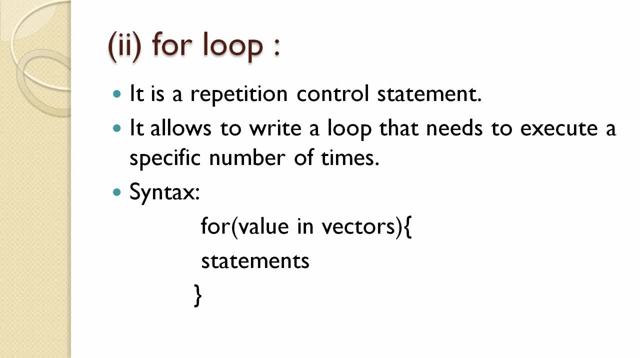 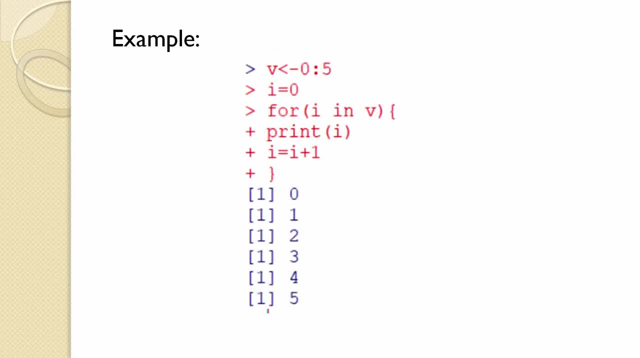 of value in vectors, which means until a value exists in the vector. we have given the condition of value in vectors, which means until a value exists in the vector, the for loop statements will be running or repeating it themselves. if we see an example: we have assigned a variable v with value 0 to 5and also a variable i equal to 0. now we 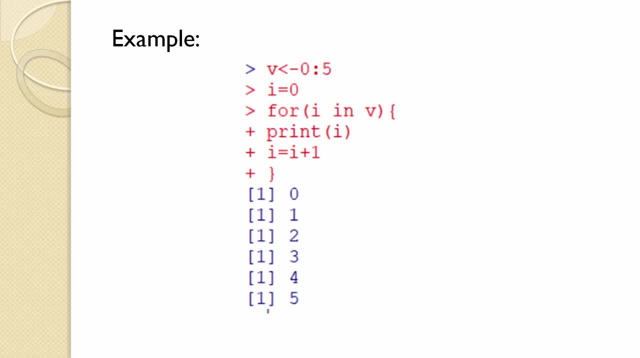 we have written a for loop for i in v, which means i values until present in vector v. i values until present in vector v. the statements inside the for loop will be executed. the statements inside the for loop are: print vimos, the value of print, the value of i and increase the value of настроff if aka edit and then we print. 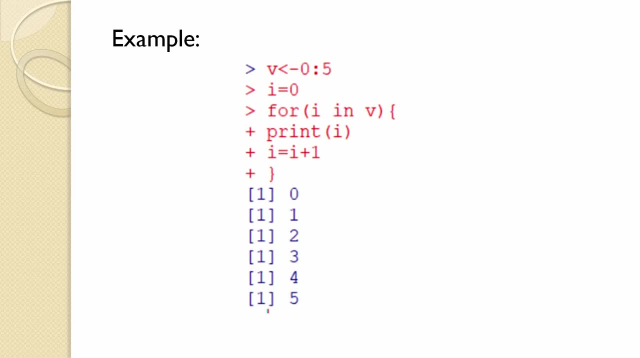 aj for for by 1.. Here we can see that initially, the value of i is 0 and 0 is present in v, which is true as it contains the value starting from 0, ending with 5.. Thus we enter into the for loop and print. 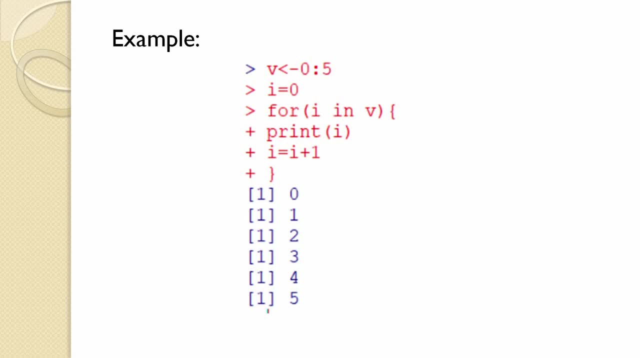 the value of i, which is 0. Then we increase the value of i by 1. The present value of i is 1.. i 1 is present in v, which is true again. Thus we go into the for loop and print the value of i as: 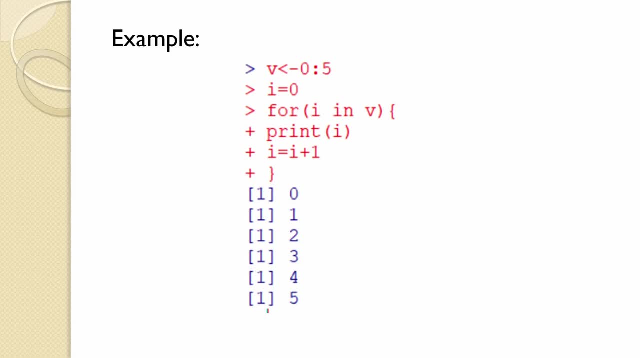 1.. Then we increase the value of i with 1 again, which means the present value of i is 2.. As 2 is also present in vector v, we again enter into the for loop and print value 2 and increase the i value as 3.. As 3 is also present in v, we print the value 3 and increase. 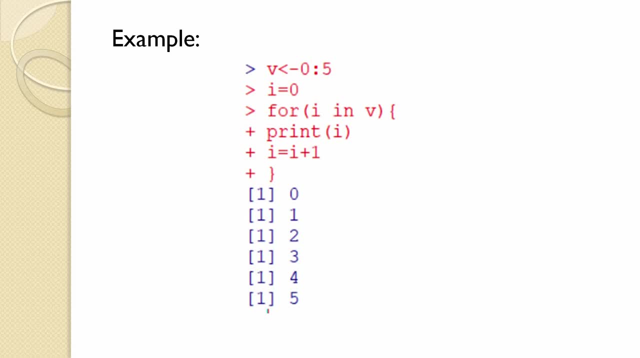 the value of i by 1, which means i value is 4.. As 4 is also present in v, we again go into for loop and print the value 4 and increase the value with 5.. Now, as the present value of i is 5 and 5 is also present in, 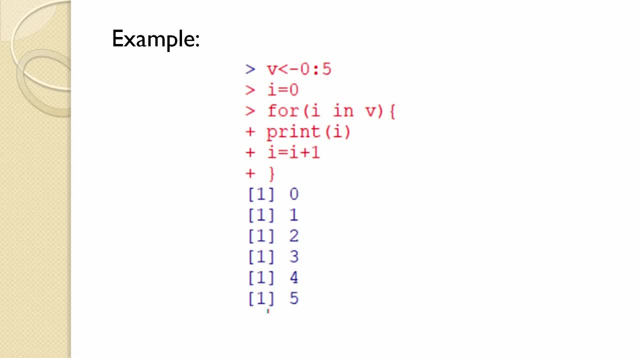 vector v. Thus we again enter into the for loop and print the value 5 and increase the i value by 1, which is i equal to 6.. As 6 is not present in v, thus the condition of i in v becomes false, and 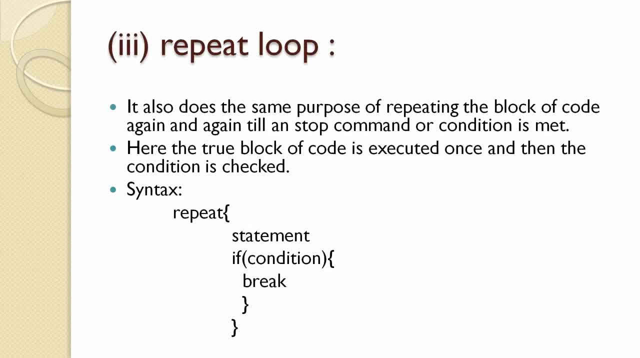 program exits the for loop. The next condition is repeat loop. It also does the same purpose of repeating the block of code again and again till a stop command is met. Here the only difference is in previous while and for loop. only after checking the condition the true statements are executed, But in repeat loop at. 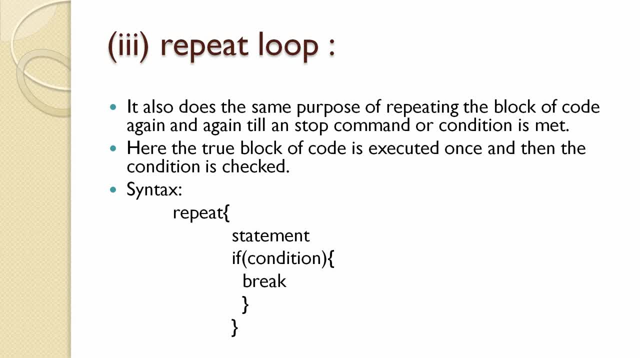 least. once the true statements are executed, then the conditions are being checked. Here we can see the syntax repeat which contains the true block statements. After these statements are executed once, then the condition is checked with if statement. if the condition is true, then we would break the loop, and if the condition is false, we would again check for the condition to be true. 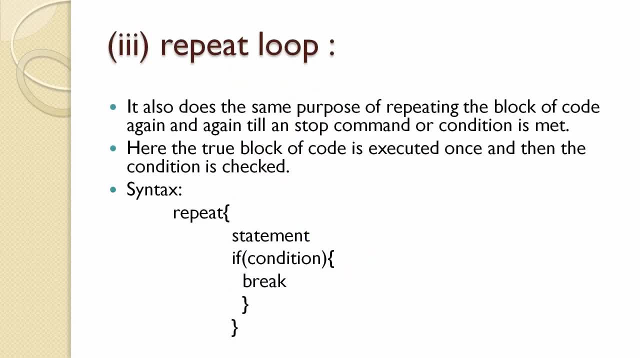 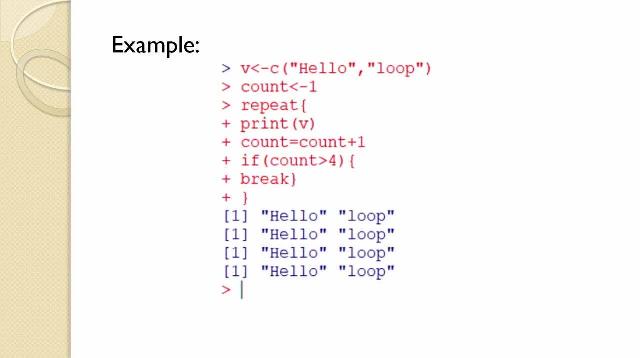 In the syntax we can see that the repeat keyword is used and within it the true statements which are to be executed are executed once before checking the statement and then by using: if we check the statement and accordingly the repeat is used, statements are repeated. if we see an example: we have done a variable v with a vector which. 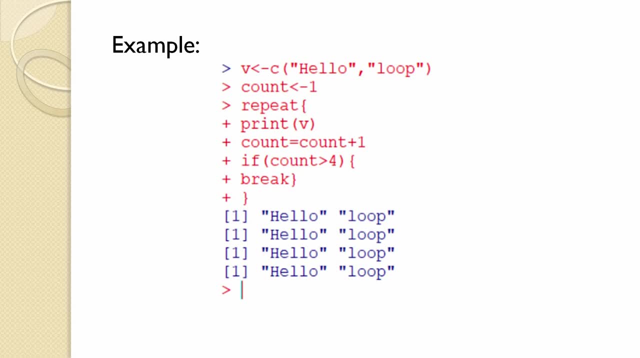 contains an elements hello and loop and also variable count is assigned with a value 1. we have started the repeat loop in which the true statement, which is to print v, which is hello loop, is executed first and the value of count is increased by 1 and then the condition is checked. 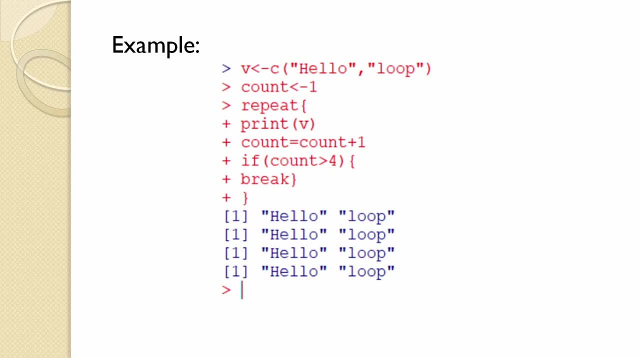 whether count is greater than 4 or not. if the count is greater than 4, then a break statement is to be executed. that exits the loop. here the value 1 is greater than 4, which is false. thus we repeat the loop and print hello loop and increase the value of count by 1. 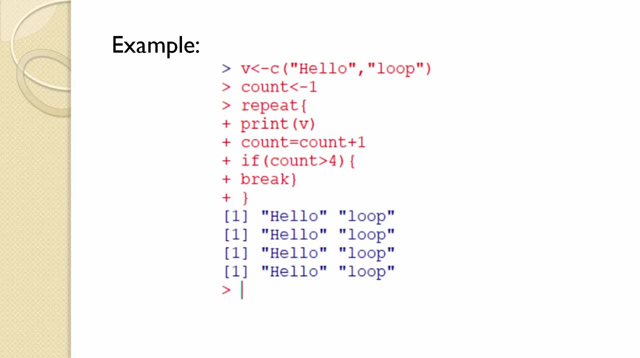 which means the present value of count will be 2. again, 2 is not greater than 4. thus we again repeat the loop and print hello loop and increase the value of count by 1, which means the present value of count is 3.. As 3 is greater than 4, condition is false. 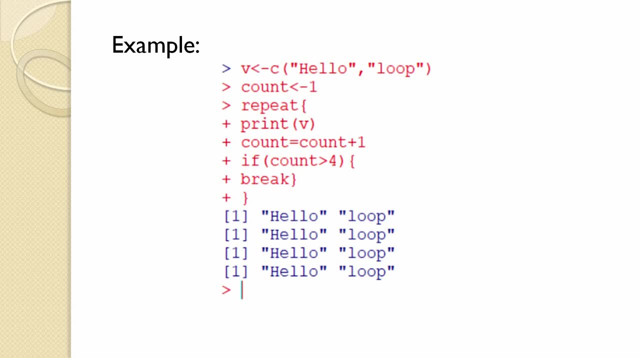 thus we again repeat the loop print v, and increase the value of count by 1. thus the present value of count will be 4.. If we again check the condition whether 4 is greater than 4, which is false, thus we again repeat the loop hello loop and increase the value of count by 1, which is 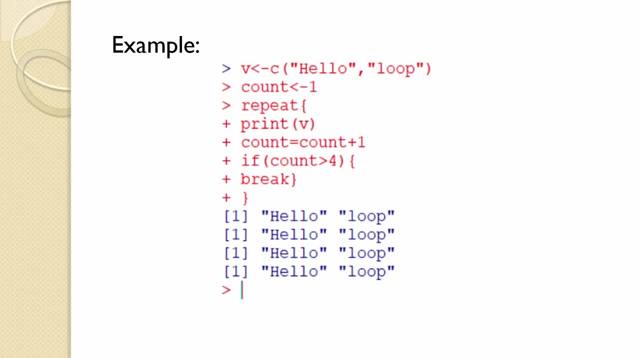 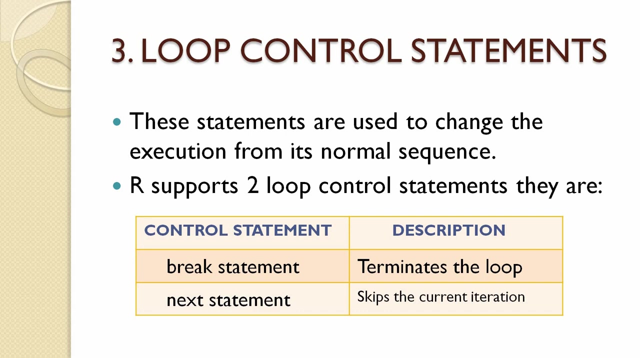 5. As 5 is greater than 4 is true. thus the program enters into the if statement block and executes the break statement and exits the entire repeat loop. The next concept of control structures are loop control statements. These are the statements which are used to change the execution of the 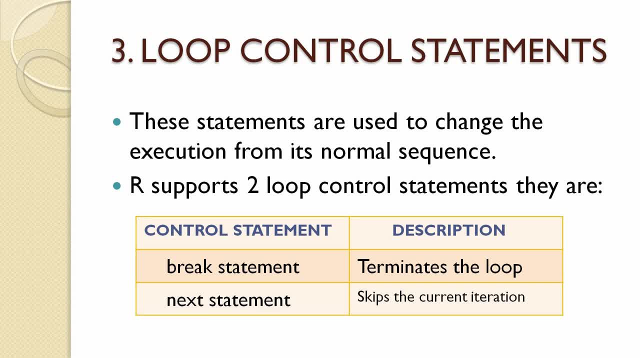 program from its normal sequence Here. r supports two loops control statements. they are break and next statement. the break statement is used to terminate the loop, which means to end the loop when a condition is satisfied and the next statement skips the current iteration if the condition 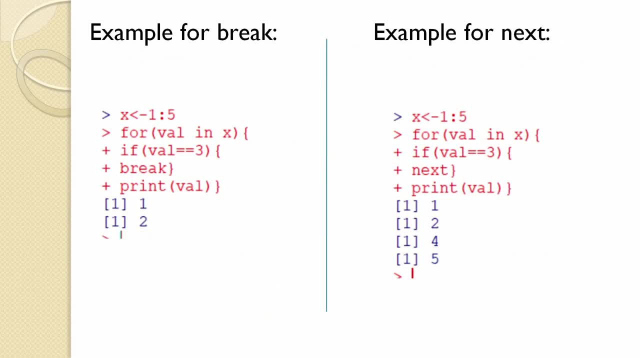 is satisfied. We can understand about this by looking at the example. If we see, for the example of break we have assigned a variable x with values 1 to 5 and a for loop is used to check for the variable val, whose initial value is 1, is present in x or not. If 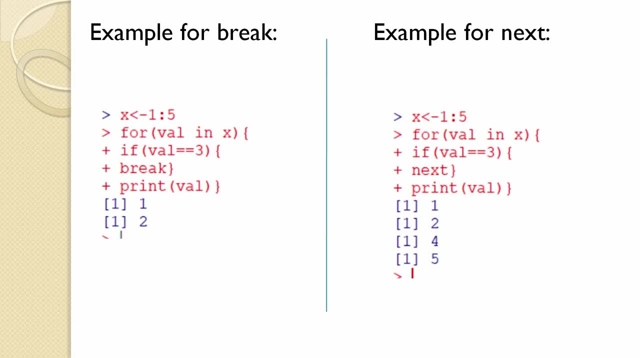 it is true, then we would enter into the for loop and the value of variable val is equal 3. thank, Then we will execute the break statement. as 1 is not equal to 3, we print the value of val and again checked for variable to. As 2 is also not it equal to 3, we again exit if statement and print the value to. 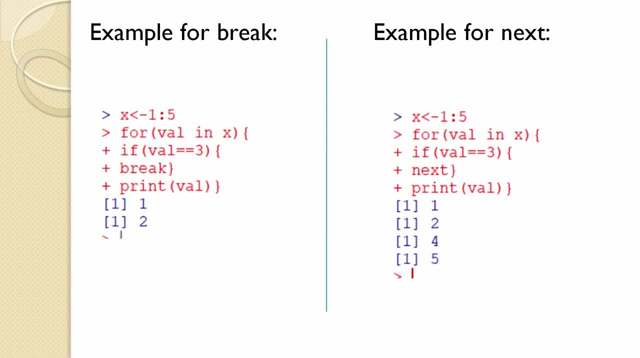 After increment again, the value of variable val is equal to 3.. the if condition becomes true and the break statement gets executed and the entire program exits the for loop. in the same example of next next statement we have taken the variable x with the values 1 to 5, and for a variable with name, val, whose initial value is 1, we are checking: